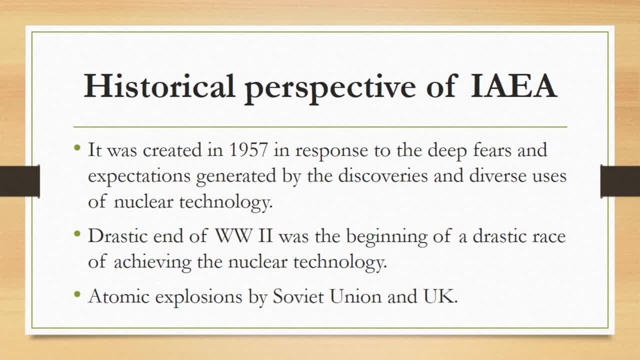 against Japan, after which the World War II was ended. The drastic end of World War II was the beginning of a drastic race of achieving the nuclear technology. Big actors of the World War II considered it their most important priority to achieve the nuclear technology, as nuclear technology had emerged as the most powerful and decisive. 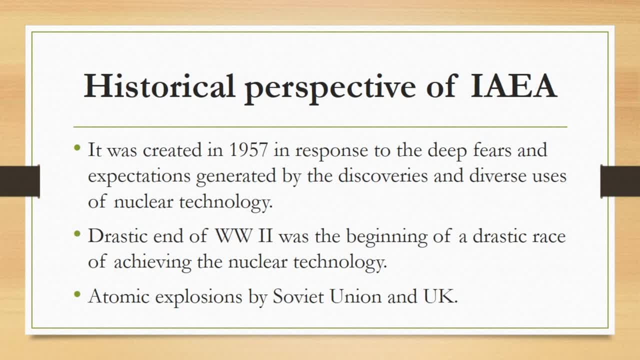 technology. at that time, Countries started fast research in this regard and opened the avenues for the nuclear proliferation. Just four years of first use of nuclear weapons by the United States, the Soviet Union conducted its first nuclear test explosion in 1949.. The first nuclear test explosion in 1939.. 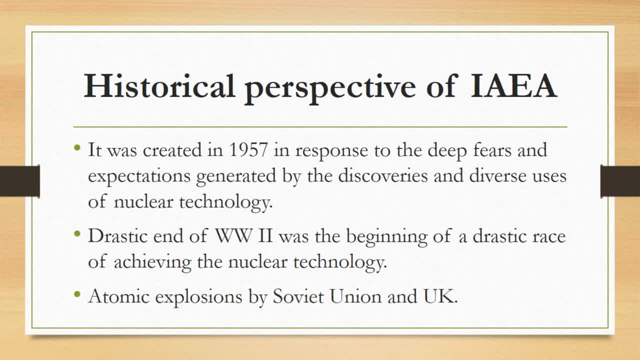 The first nuclear test explosion in the United States. The first nuclear test explosion in the United States. Similarly, the United Kingdom got nuclear power in 1952.. After this development, the voices against the seriousness of this race were raised. World had come to know at that time that if this process would not be stopped, then the 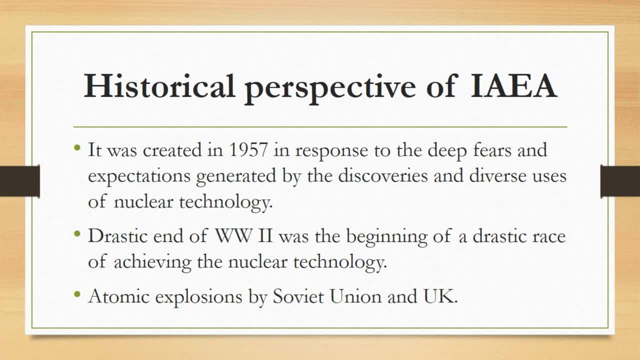 whole world may got this technology and world would be blown up any time. as world had witnessed the damages caused by the first use of nuclear weapons by the United States against Japan at the end of World War II, Some steps taken immediately to stop this race. 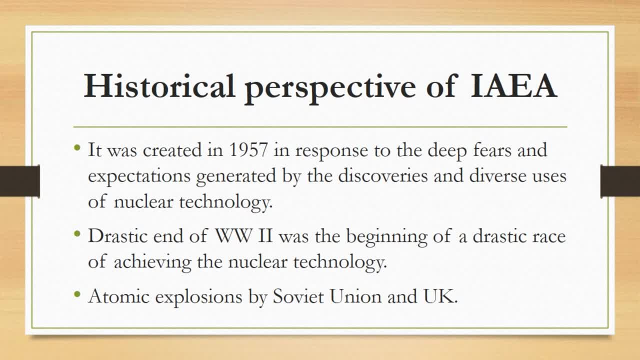 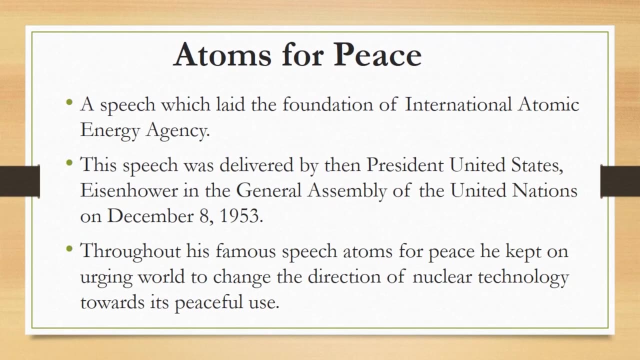 The establishment of International Atomic Energy Agency was the most important step which was taken at that time to turn the nuclear technology towards the peaceful uses Atoms for Peace. Atoms for Peace was basically a slogan Speech which laid the foundation of International Atomic Energy Agency. 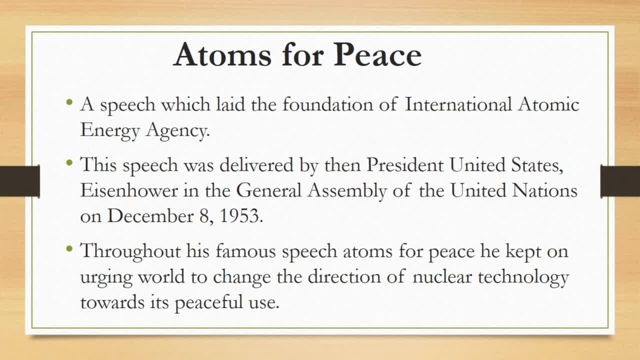 This speech was delivered by then President of United States Eisenhower in the General Assembly of the United Nations on December 8, 1953.. Eisenhower was a military man, a former World War II commander, drafted into a presidential campaign. He entered office in 1953 as the first chief executive elected after the advent of the. 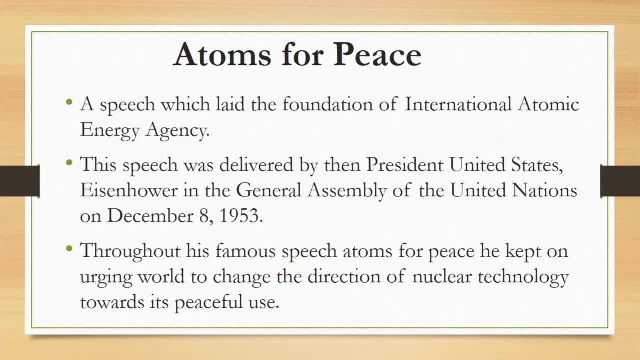 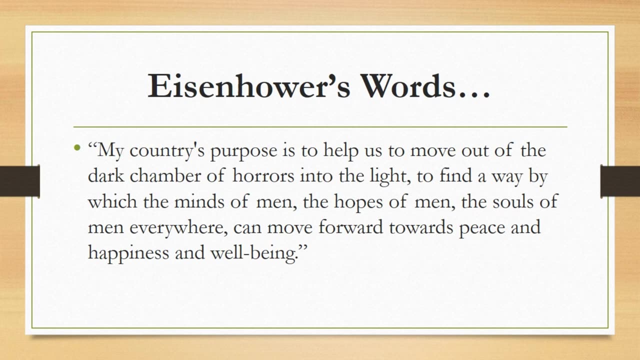 bomb. Throughout his famous speech Atoms for Peace, he kept on urging world to change the direction of nuclear technology towards its peaceful use. He said: My country's purpose is to help us to move out of the dark chamber of horrors into the 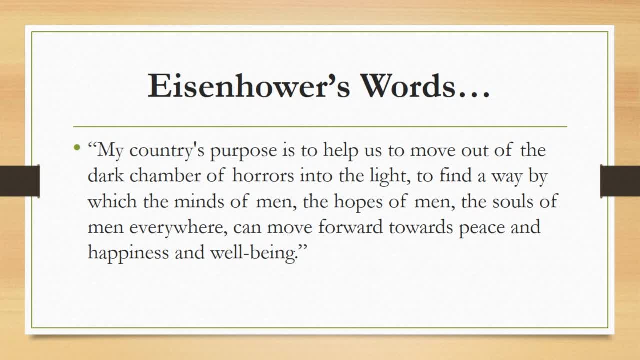 light to find a way by which the minds of men, the hopes of the men, the souls of men everywhere can move farther. He said I will continue to move forward towards peace and happiness and well-being. During his speech he gave proposal for an agency to promote peaceful use of nuclear. 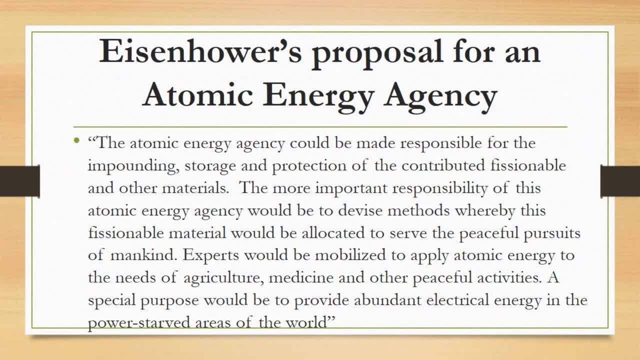 technology. His exact words were: The Atomic Energy Agency could be made responsible for the impounding, storage and protection of the contributed fissionable and other materials. The more important responsibility of this Atomic Energy Agency is to protect the environment. Atomic Energy Agency is responsible for the protection of the contributed fissionable and. 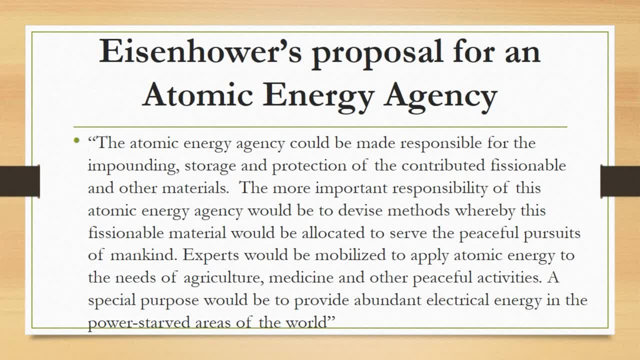 other materials. The agency would be to devise methods whereby this fissionable material would be allocated to serve the peaceful pursuits of mankind. Exports would be mobilized to apply atomic energy to needs of agriculture, medicine and other peaceful activities. A special purpose would be to provide abundant electrical energy in the power-starved areas. 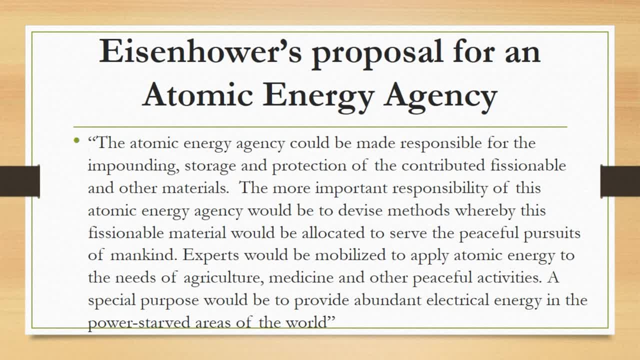 of the world. So these were the words of Atomic Energy Agency, These were the words of Eisenhower, through which he gave the proposal of the establishment of International Atomic Energy Agency, which came into being in 1957 on the basis of this Speech, which is titled as Atoms for Peace. 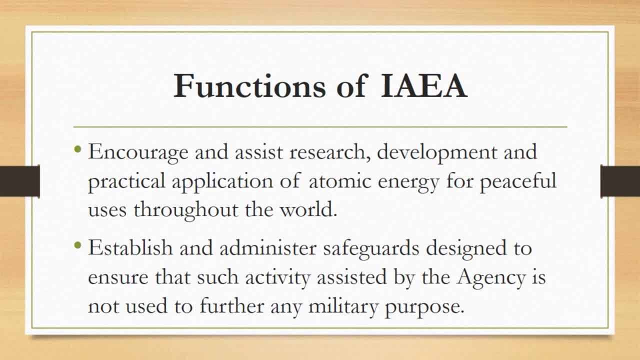 Functions of International Atomic Energy Agency. The main function of the IAEA are to encourage and assist the people, the community and the institutions to achieve peace and prosperity. The main functions of IAEA are to encourage and assist the people, the communities and. 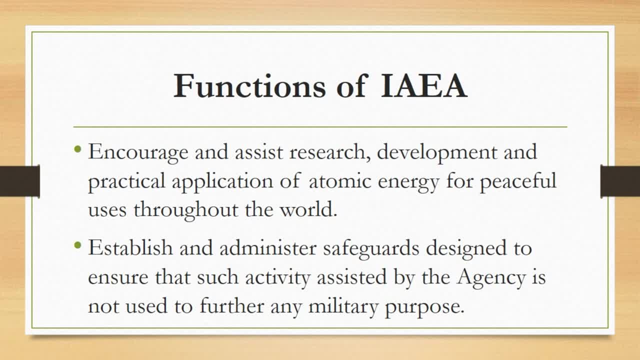 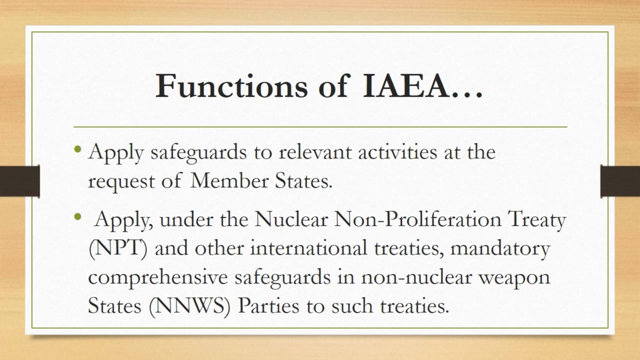 assist research, development and practical application of atomic energy for peaceful uses throughout the world. Establish and administer safeguards designed to ensure that such activity assisted by the agency is not used to further any military purpose. Apply safeguards to relevant activities at the request of member states. 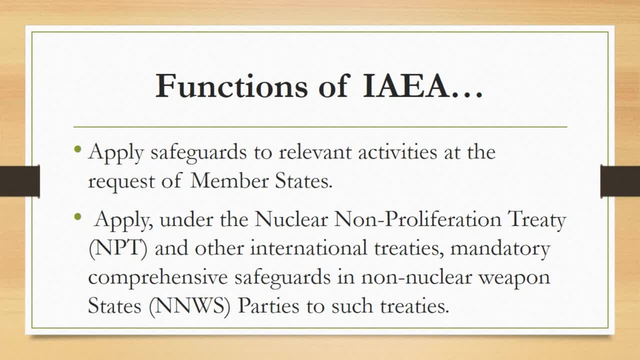 Apply, under the Nuclear Non-Proliferation Treaty and other international treaties, mandatory comprehensive safeguards in non-nuclear weapon states parties to such treaties. In carrying out its functions, the agency conducts its activities in accordance with the purposes and principles of the United Nations Charter to promote peace and international. 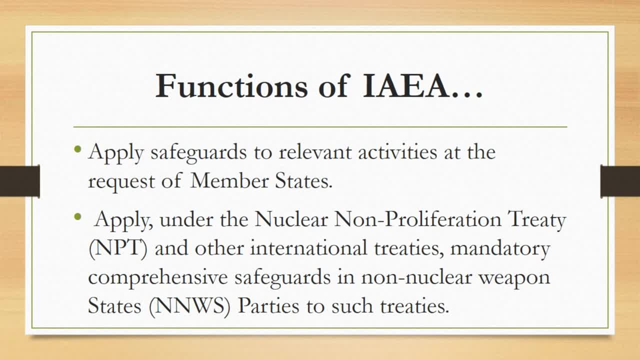 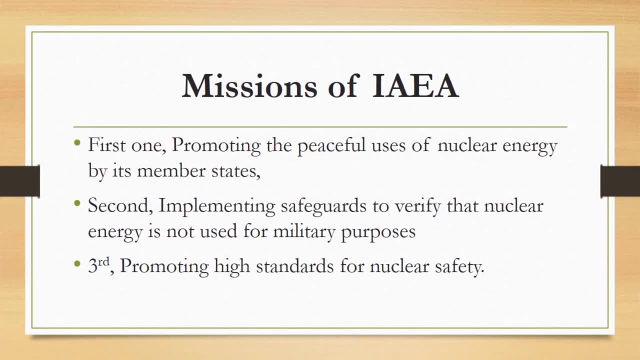 cooperation and in conformity with policies of the United Nations For furthering the establishment of worldwide disarmament through safeguards Missions of IAEA. The International Atomic Energy Agency is generally described as having three main missions. First one, promoting the peaceful uses of nuclear energy by its member states. 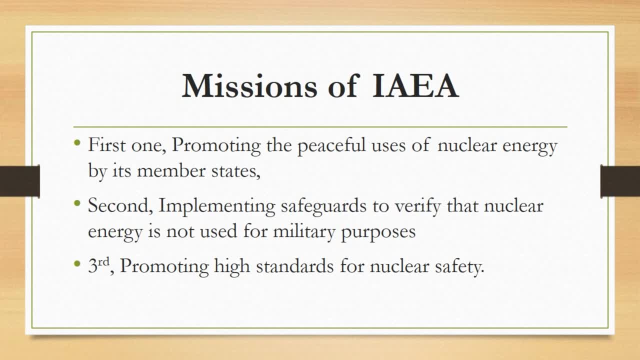 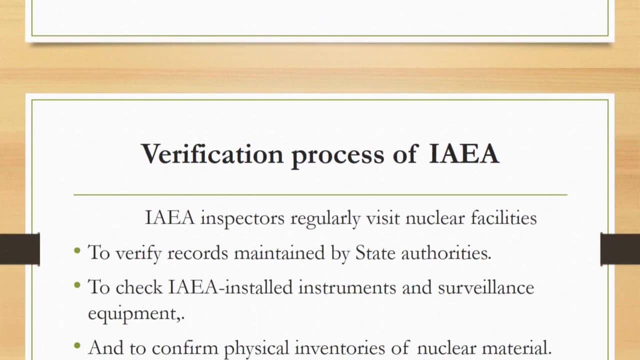 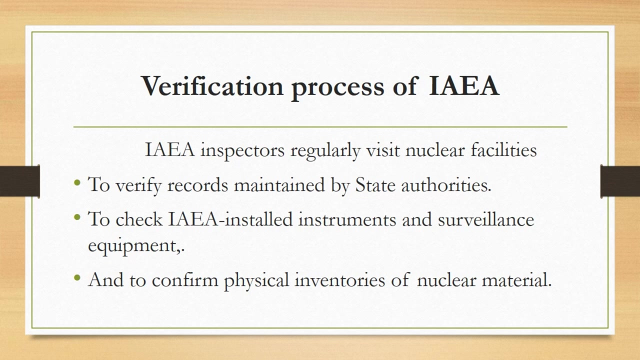 Second, implementing safeguards to verify that nuclear energy is not used for military purposes. And third one, promoting high standards for nuclear safety. Now, what is the verification process of IAEA? Under Safeguards Agreements, IAEA inspectors regularly visit nuclear facilities to verify. 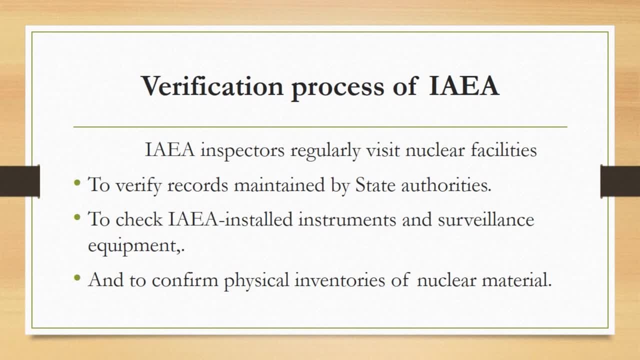 records maintained by the state authorities on the whereabouts of nuclear materials under their control, To check IAEA installed instruments And surveillance equipment And to confirm physical inventories of nuclear materials. These and other safeguard measures provide independent international verification that governments are abiding by their commitments to the peaceful use of nuclear technology. 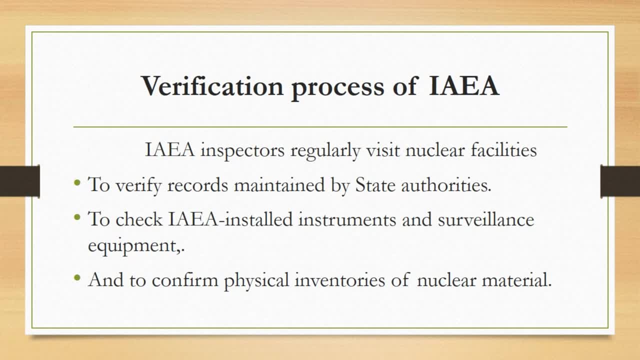 A precondition for the implementation of safeguards is a formal safeguards agreement between the agency and the state. The regulations are very simple and the IAEA does not deal with any of these. There are five types of inspections under IAEA. There are four types of inspections under IAEA. 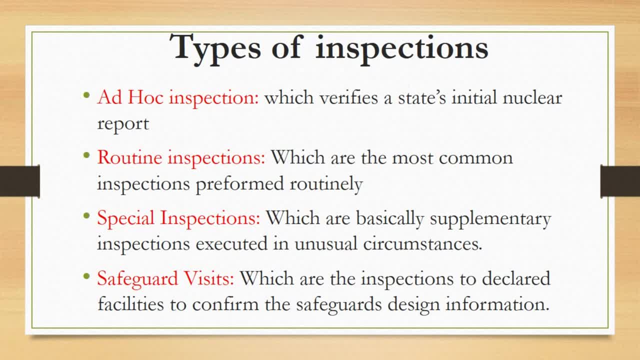 Ad-hoc inspection, which verifies a state's initial nuclear report. Routine inspections, which are the most common inspections which are performed routinely. Special inspections, which are basically supplementary inspections executed in unusual circumstances. Or special inspections which are performed with special permission for the purpose of